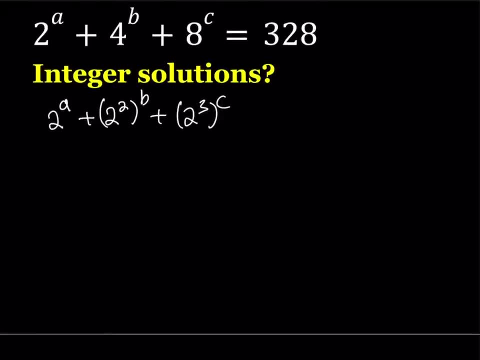 I'll write it. I'll set it equal to 328.. Okay, so, from power of a power rule, we can just go ahead and multiply the these exponents: 2 to the power 2b or not 2b. Finally, I got that 2 to the power 3c and that is equal to 328.. So what am I going to do with? 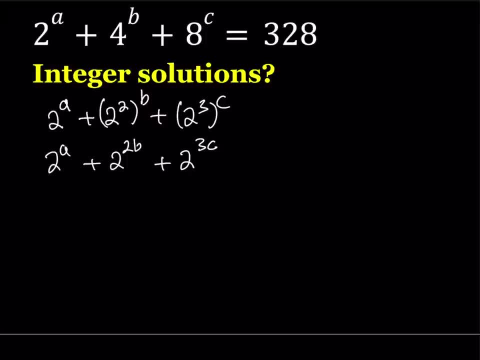 this expression. First of all, they are all different powers. One of them is a multiple of 2,, one of them is a multiple of 3, so on and so forth. So this is what I'd like to do. I'd like. 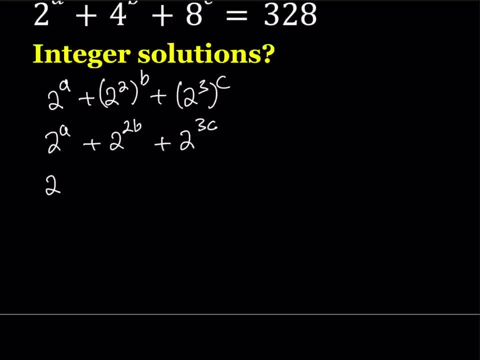 to factor out something, because a lot of times with exponential equations, factoring helps. So let's go ahead and take out 2 to the power a, and now what happens is this becomes 1,. this becomes 2 to the power 2b. 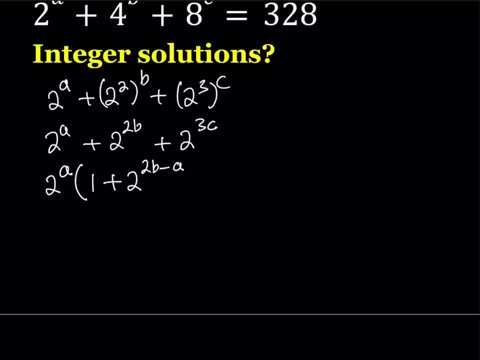 Or not. 2b minus a- Okay, I'm overdoing it, sorry- Plus 2 to the power. 3c minus a. Okay, now notice that I made an assumption that 2b minus a is going to be a positive, which means 2b is greater. 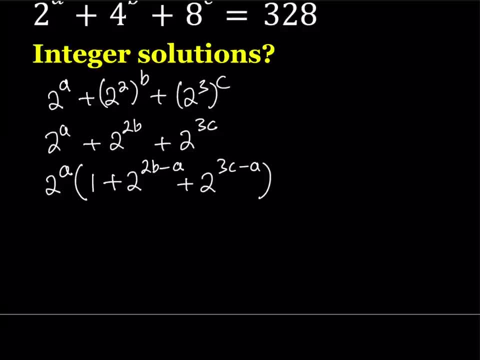 or equal to a, which. if that doesn't work, we're going to get a fraction from here and things are going to be messed up, But you'll see that it's going to work. So this is equal to 328, and what I can do is, at this point, I can factor 328 as well. So let's go ahead and factor it. 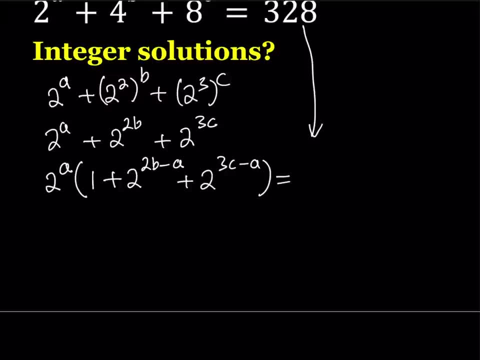 I can write it that way: 328 can be written as 8 times 41, which is equal to 2 to the power, 3 times 41.. Now, one of the nicest things about 41 is that 41 is a prime number, so there's no way it. 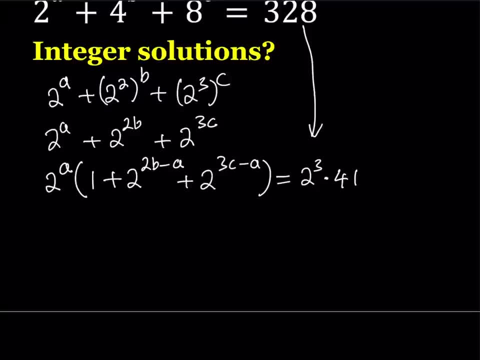 can be equal to a power of 2 and 2 to the power a must equal 2 to the power 3.. So from here we get that a is equal to 3.. That's one of the conclusions we're getting. What about the other one? Well, we. 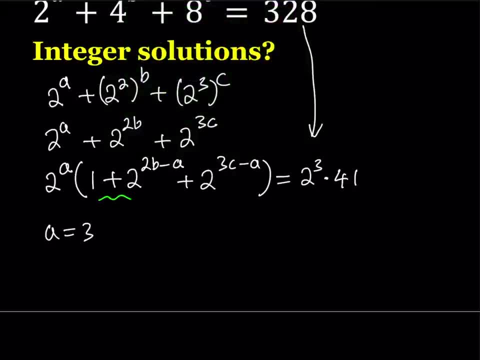 can also say that we can also say that this piece here is going to be equal to 2 to the power 3.. Since 2 to the power a is equal to 2 to the power 3, this piece must equal 41. But that implies that 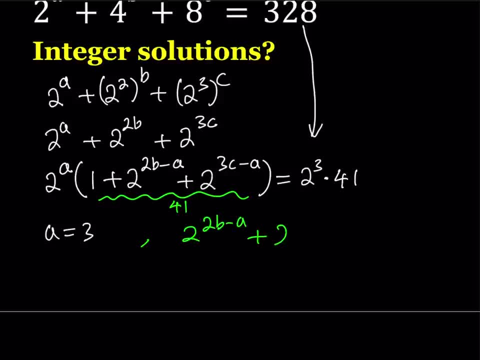 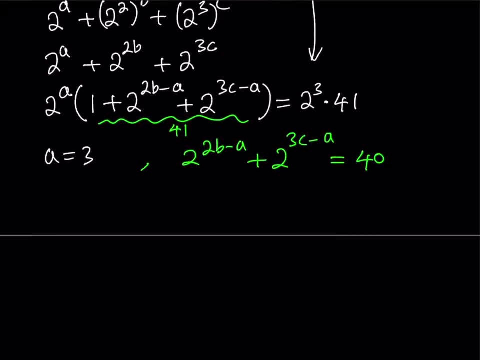 2 to the power 2b minus a. plus 2 to the power 3c minus a is equal to 41 minus 1, which is 40.. Now one of the nicest things about this equation is that once you simplify a little bit, like I got, 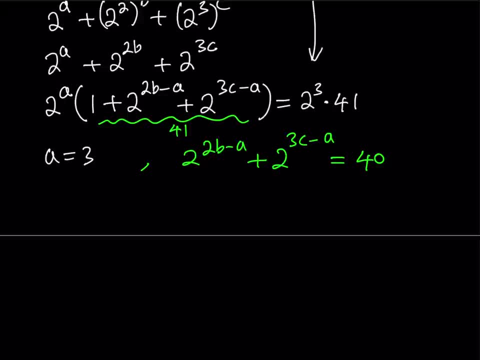 an idea about a. I can go ahead and simplify this even more by factoring again, But I'm going to factor the right hand side. So instead of 40, I can just write 8 times 5.. Which can be written as 2 to the power 3 times 5.. Right, And what is so cool about it? Now notice. 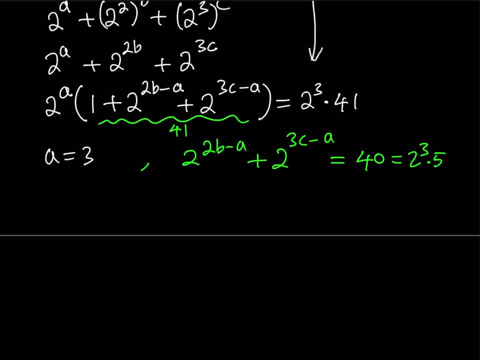 that on the left hand side we have the sum of powers of 2.. On the right hand side, we have a product. So why don't we just try to write it as a sum of 2 powers of 2.. And we can do that actually. 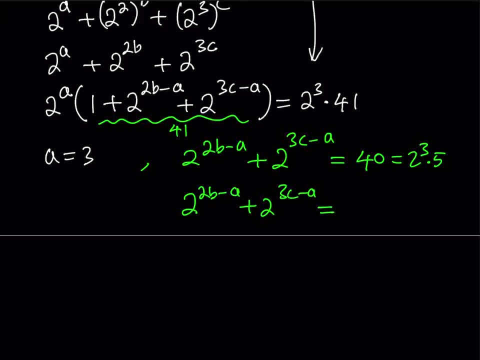 if you notice that 2 to the third power times 5.. So 5 can be written as 4 plus 1, which is a power of 2, by the way, And if you write it as 2 squared plus 1. And distribute to 2 to the third, you're basically going to be getting what you need, And that is. 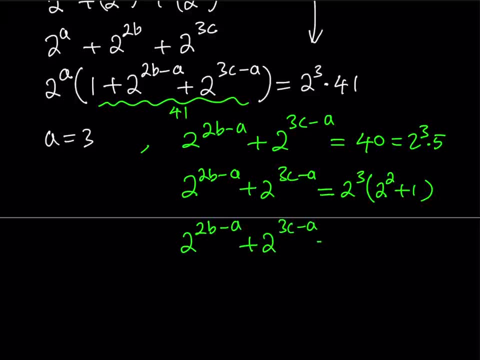 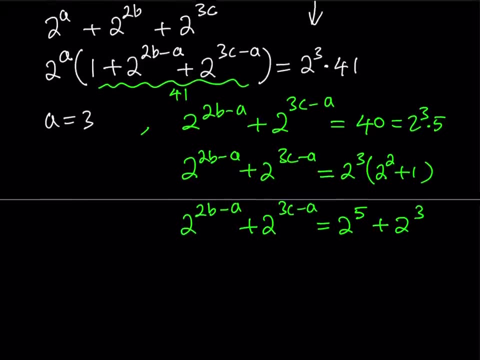 being able to write it as a sum of powers of 2.. So from here we get 2 to the fifth power, plus 2 to the third power. Great, So this is a really nice equation, because a, b, c are integers and 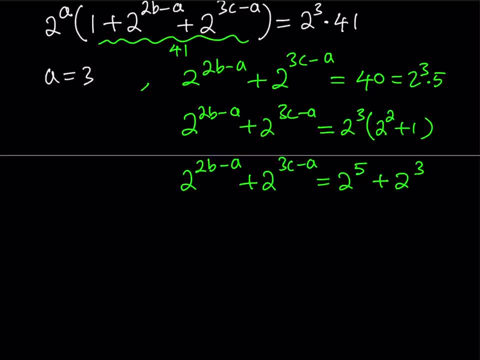 I already have a value for a And we're going to look into other values of a if possible. Or you can just argue that is there going to be a possible value of a? Probably not Right. Anyways, let's continue. So from here we get two cases. So what are those cases? Well, first case is, first of all, 2b minus a. 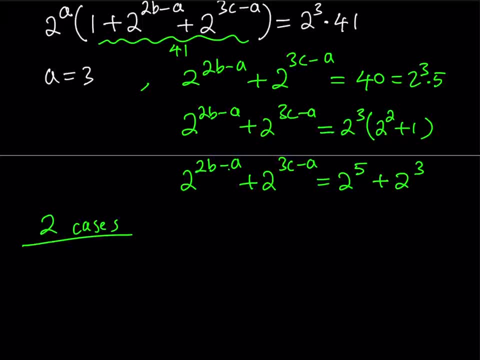 can equal 5.. And the other one can equal 3, or vice versa. So let's go ahead and take a look at each case. So 2b minus a can equal 5. And 3c minus a can equal 3.. Because we have these exponents and 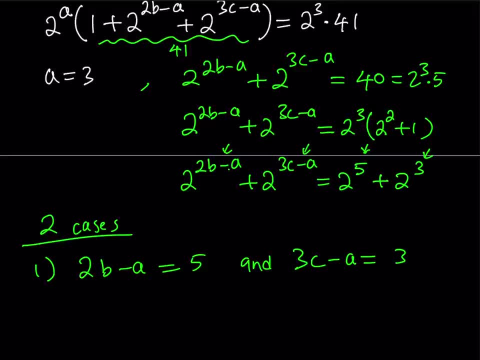 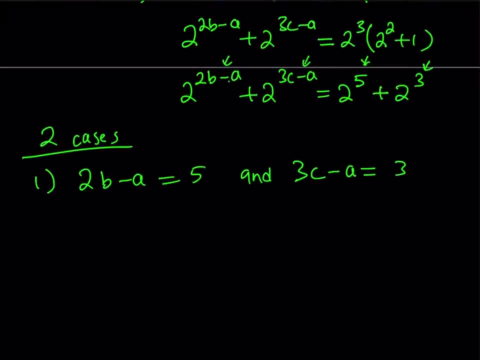 we have those exponents And, obviously, since these two sums are equal to each other, Is there a way to that? they're not going to be equal to each other, But two different powers of 2 they're going to add up to give us the same number. Is that going to be possible? Something to think about, Okay, Anyways. 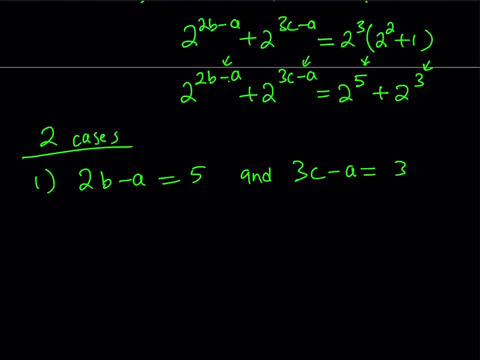 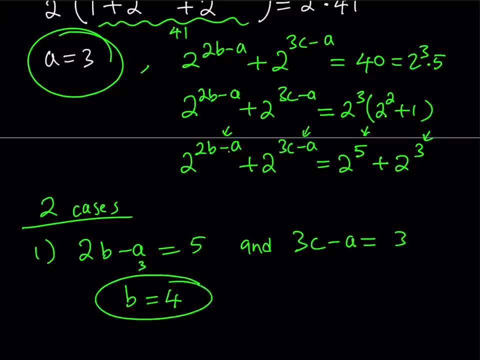 let's just proceed with this one From here. since we already know that a is equal to 3, we can just go ahead and substitute that 2b equals 8.. That's going to give me b equals 4.. And if I plug in, 3. 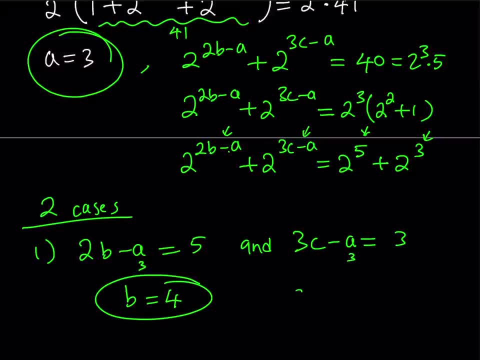 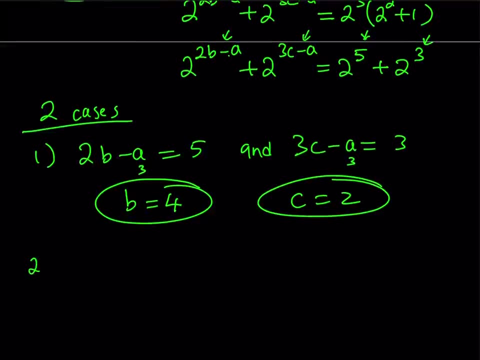 here, 3c equals 6 is going to give me c equals 2.. And that is going to be a valid value. So we're going to have a valid solution. obviously, Right. But let's go ahead and take a look at the second case and see. 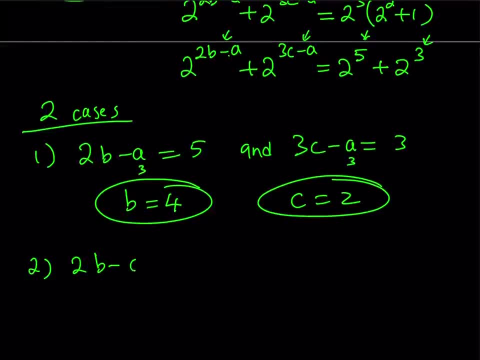 what that gives us. So we're going to switch around: 2b minus a is going to be 3. And 3c minus a is going to equal 5.. Is that possible? So that's what we're going to check next, And if that works, then 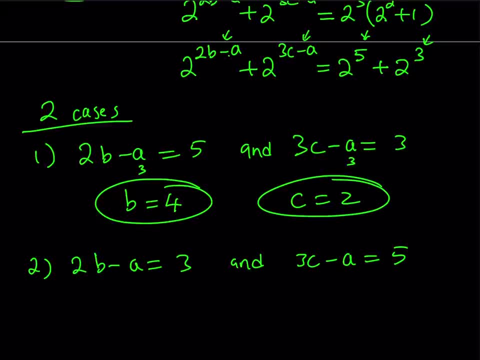 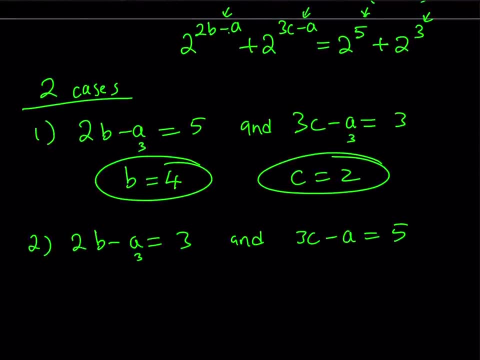 we'll get another solution And we'll just put it all together. Okay, Since a is equal to 3.. Remember, we've found that previously. From here we get 2b equals 6. Which means b is equal to 3. So 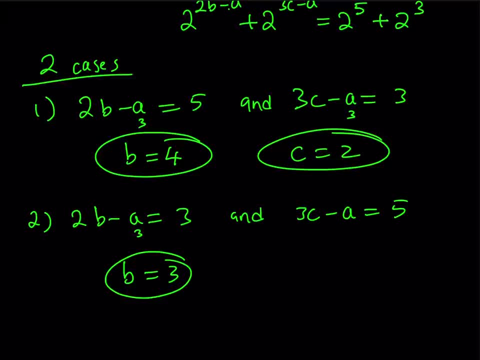 that looks like a good solution, But let's go ahead and check for c as well. Now, if c is equal to well, I shouldn't say c. If a is equal to 3, then we get 3c equals 8.. But unfortunately this does. 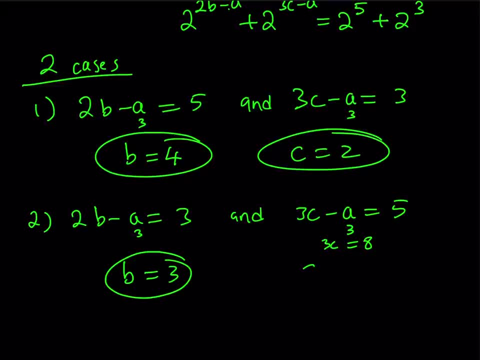 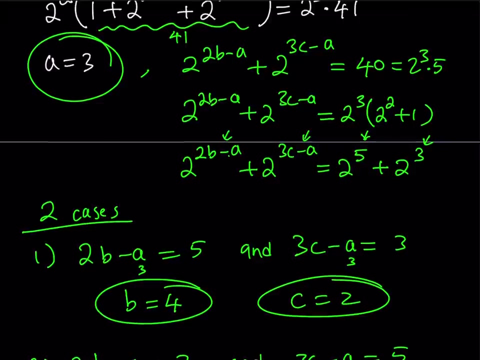 not give us any integer solutions. So in this case c is not going to be an integer. Now what is that supposed to mean? We're not getting any solutions from the second case. Okay, Does that make sense? Hopefully that does. Now, if you put it all together, we're going to be looking at a 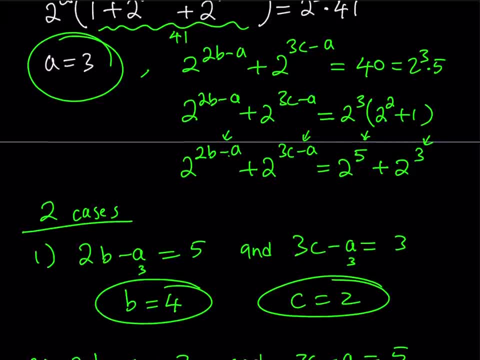 single solution here: a equals 3.. b equals 4.. c equals 2.. But is there a way that there can be other solutions? So let's go ahead and kind of take a look at that here. Well, notice that I was. 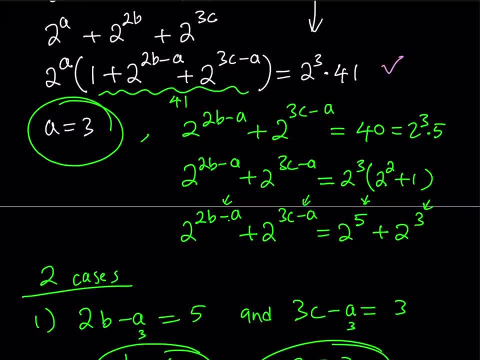 able to take out a power of 2.. But on the right hand side I do have a 41, which is a prime number, So there is no other way to simplify this. where a, b, c are integers, For example, if 2b minus a, 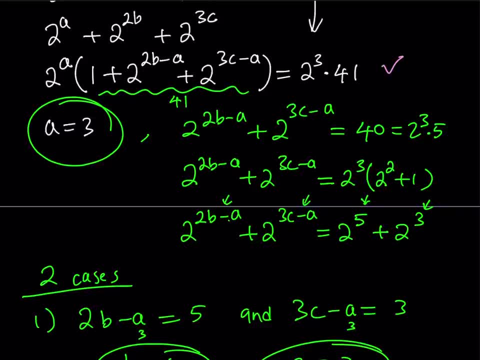 is negative, then we're going to be getting a fraction from here, But then the fraction times a power of 2 is not going to give us an integer, So we're going to be getting a fraction from here, So on and so forth. But definitely you can explore those options as well In order to 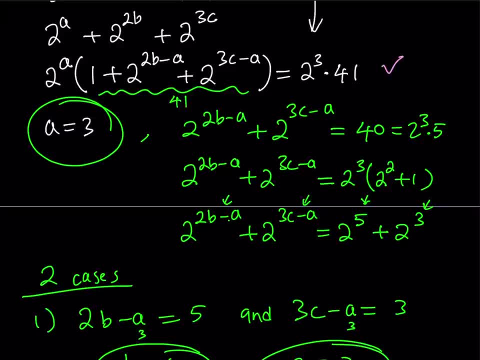 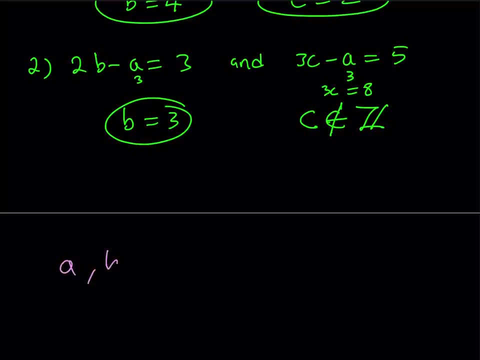 keep this video short, I'm going to skip that part, Okay. So what am I getting from here? I'm getting that a, b, c as an order, triple can be written as: And of course here we're not going to have any permutations of this, because a, b, c are fixed. If you look at the original problem, you're.